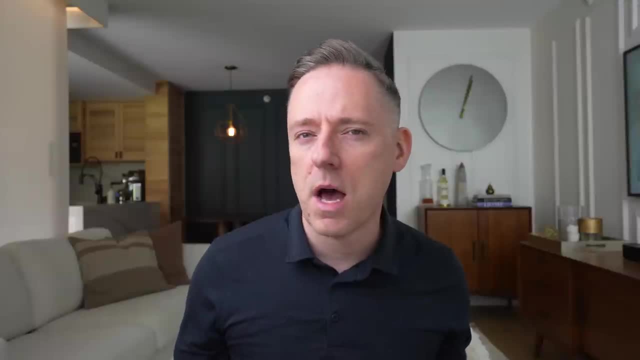 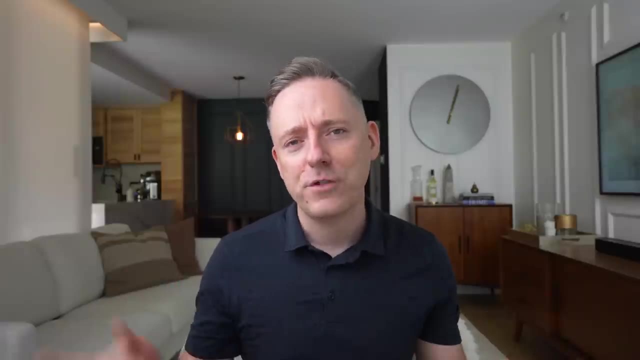 about updating it a little bit. We're just going to talk about the role of gray in interior design and have a little fun while we're doing it. So let's get to it. And first let's acknowledge my background is different. Yes, if you have been here before, I have changed my living room. 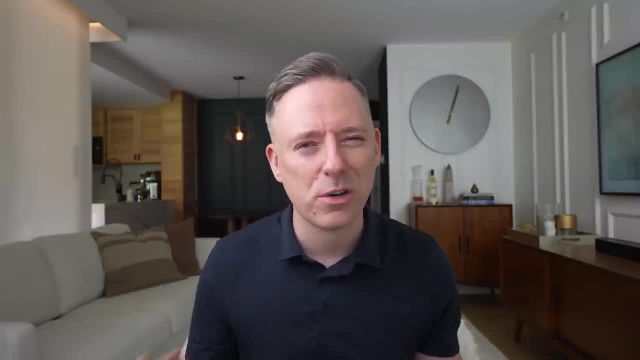 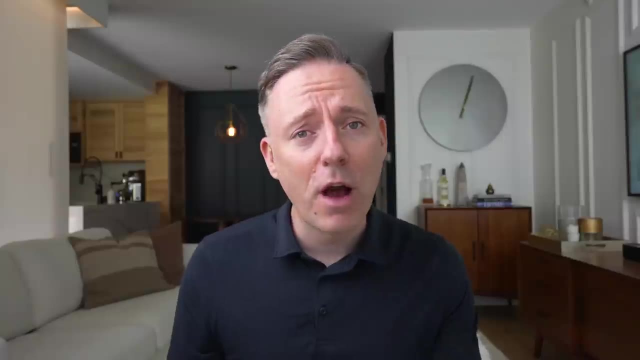 It's a whole process. I'll give you guys the whole story Once the place is done. it's all sort of trickling in. I'll give you the full story later but links are going to be down in the description as stuff trickles into my living room. If you see things in my background. 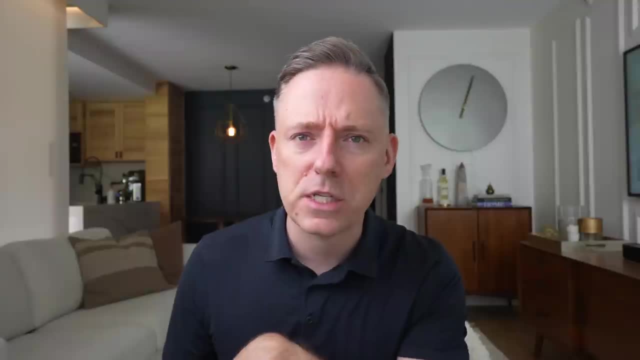 there you go. Also, my course is live by the way, Quick, shameless plug. head to the description. That's where you can check that out. Let's get to the video. Okay, so let's talk about gray a. 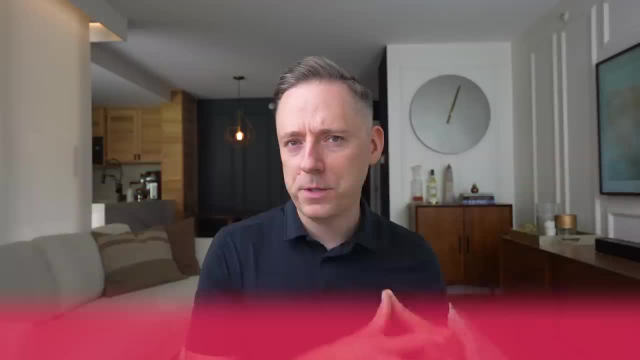 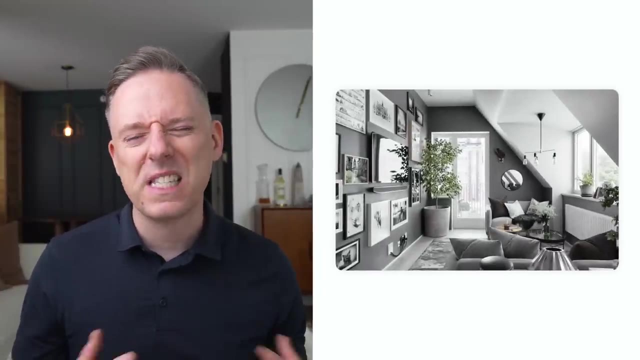 little bit because I feel like gray nowadays has a really bad reputation in interior design because people talk about sort of how it came, was so everywhere for several years and people got really sick of it because they felt it was really drab and boring and gray. 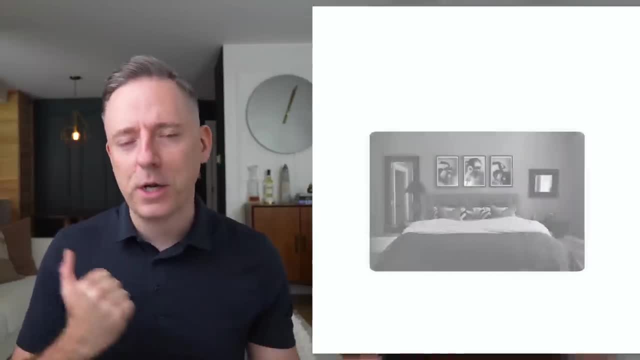 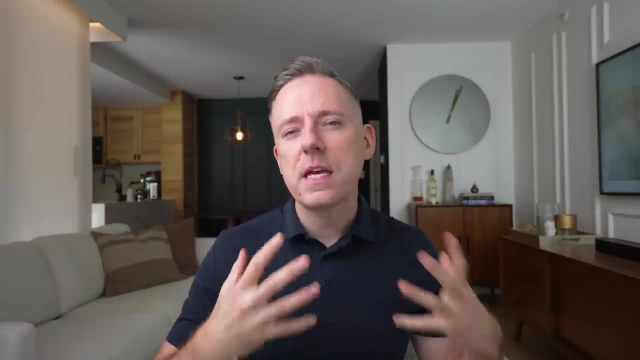 And depressing and kind of was, and that's what we're going to talk about here and maybe some ways that you can kind of fix it. But first I want to address the good qualities of gray and why it was so popular. I think the thing is with those sort of cooler gray tones is that they feel 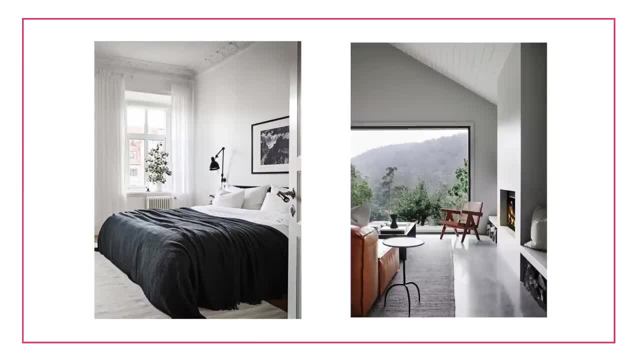 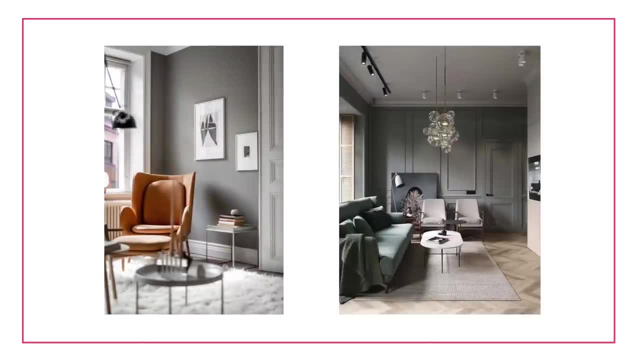 really sophisticated, They feel really chic And I think a lot of people like that. Now they do feel a little bit cold and they can feel a bit standoffish and a little bit kind of give you that art gallery effect, which is again why I think we're moving away from it, But I do think 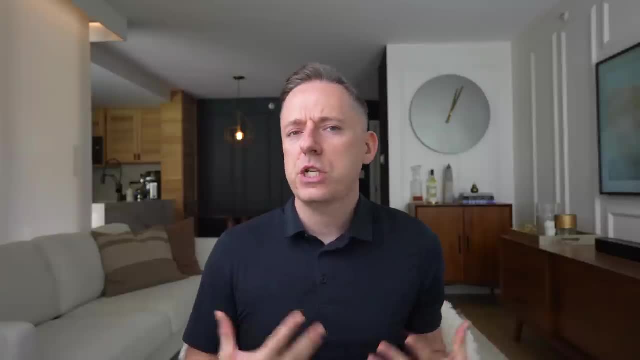 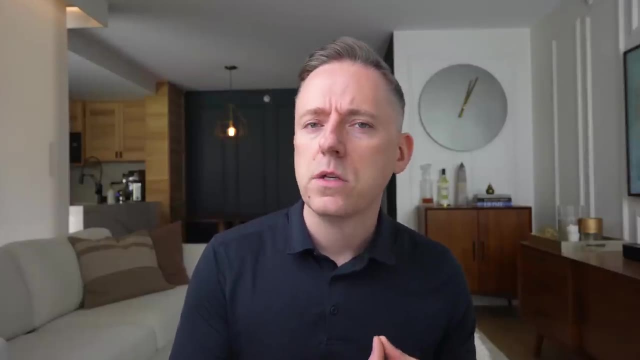 it's really popular for those reasons. It's really good at establishing a very sort of chic, sophisticated mood for a space, And I think that was really popular for a while as well. It was also sort of fit really well, I think, into styles that were really 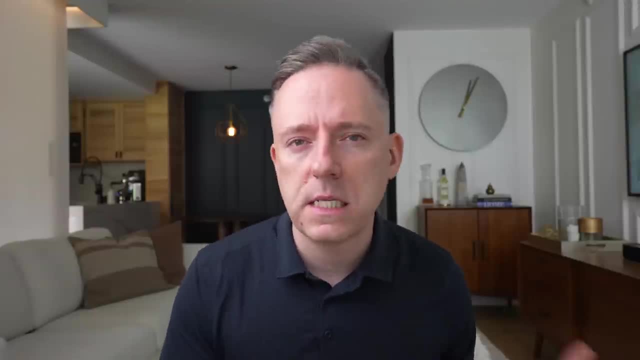 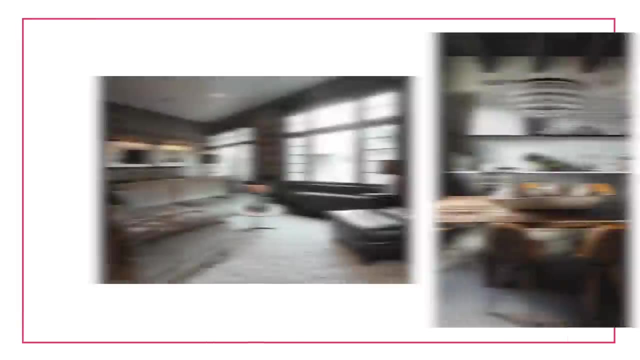 popular sort of in 2015 to 2019 sort of thing, right. So modern, farmhouse, glam, transitional spaces- I saw a lot of those spaces as being really popular and a lot of people really loved those styles and gray works really well in those styles, especially those sort of cooler tone grays. 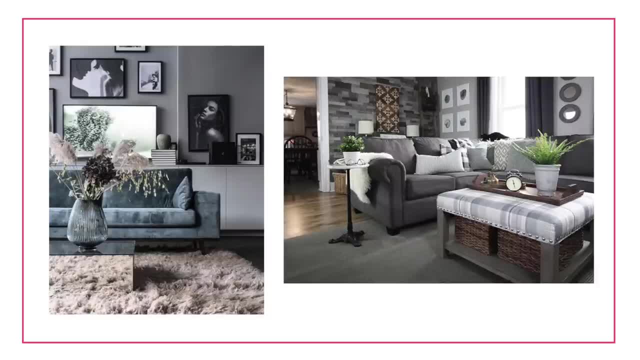 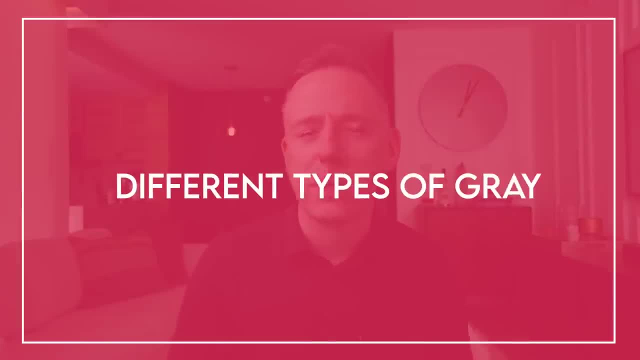 those sort of silvery, blue, grays really, really popular with those styles. And because those styles were popular, so was gray as the neutral of choice. Now I want to establish here that gray is really just a neutral And I want to really break down a little bit using the old color wheel. 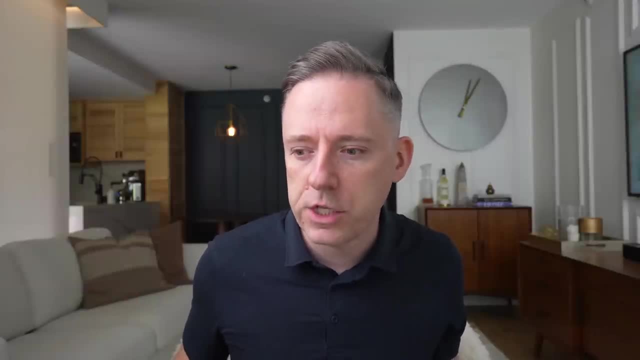 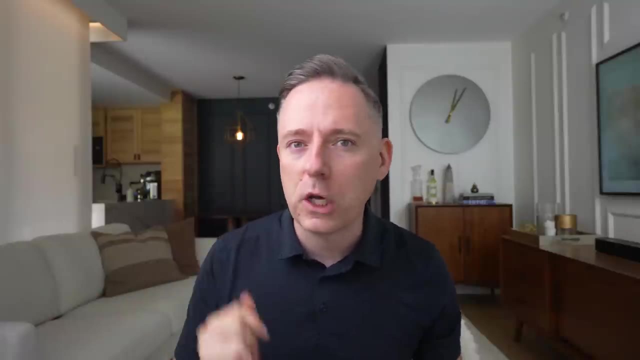 to explain sort of where gray sort of fits in all this conversation, because people have a distinct idea on what gray is. So first of all let's talk about which I've mentioned before. I have a whole video on and I'm going to link over here wherever it is called tints, tones and shades, We're 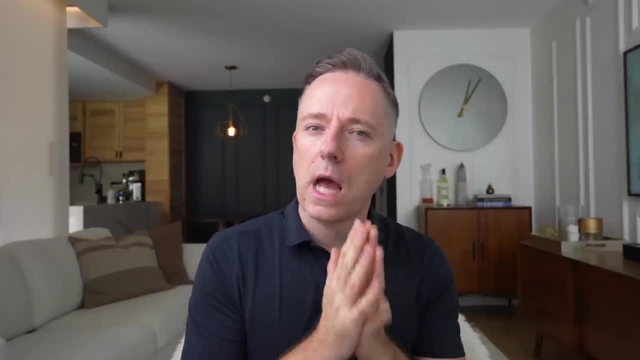 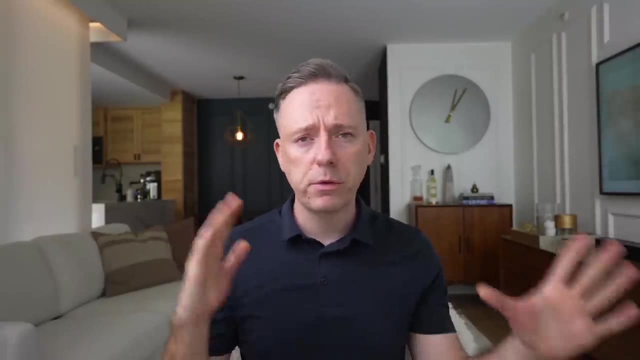 going to talk about the tints, tones and shades of different colors, because I think it's really helpful in understanding neutrals and the role of neutrals in design. So when you take a color or a primary hue could be red, whatever blue, green, what have you? 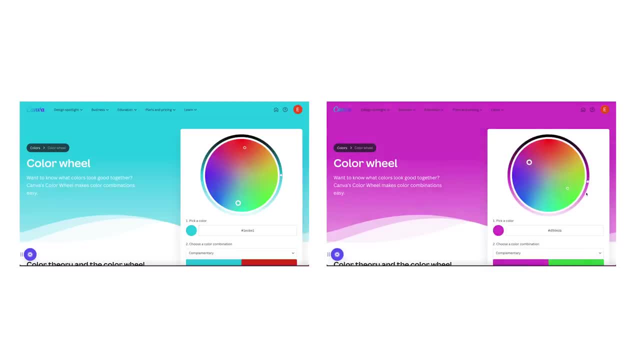 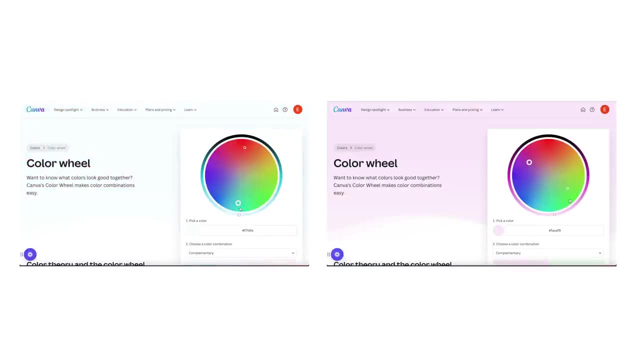 and you add a lot of white to it, it becomes a tint. It's basically becomes really, really light, And if you actually add a lot of white to it, it can basically feel like an off white or a white with a red, yellow, green, whatever sort of undertone to it. Shade is the opposite. 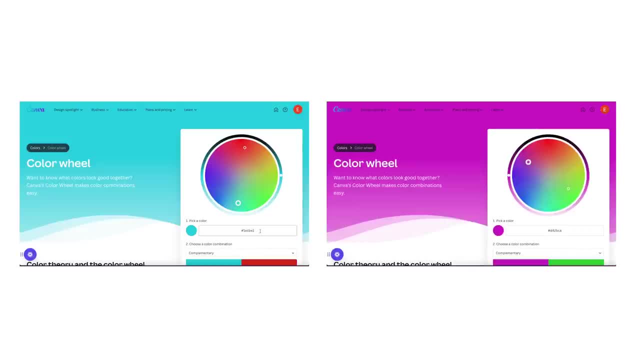 but we're adding black, So now it's going to be a darker shade of a certain color. So picture: something like blue can feel really bright and vibrant, but when you add a lot of black to it, start to read a little bit more like Navy right. 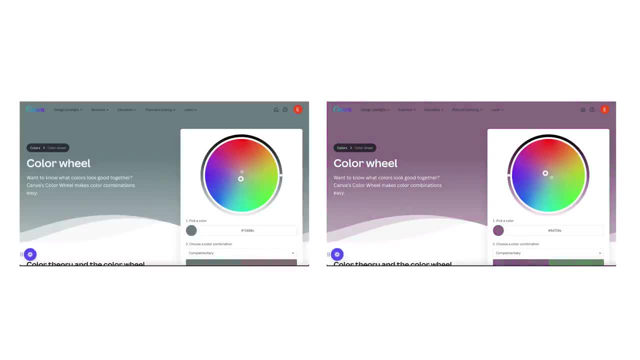 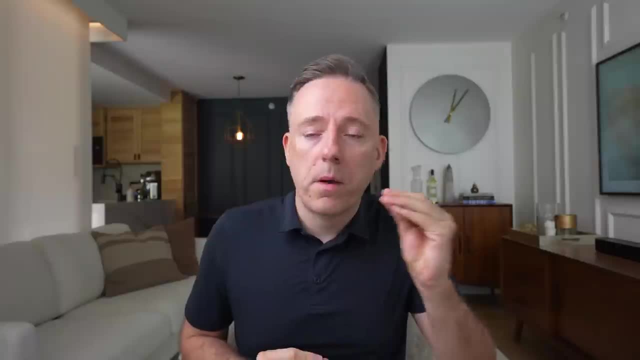 Gray, which gray is just a mix of black and white, And when you add black and white gray to a primary hue, it just sort of becomes really desaturated. And now adding different combinations of black, white and gray, two different colors, opens up the entire color. 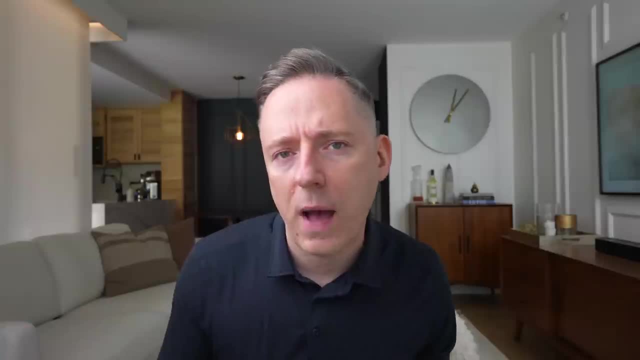 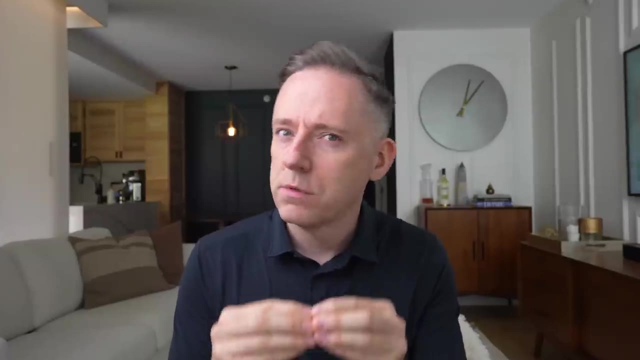 wheel to all of its splendor and all of its different options that you have. So why do I mention that in the context of gray? Because gray, when you add a lot of gray to a certain color, starts to resemble gray, but just having different undertones. And I think people think gray and the 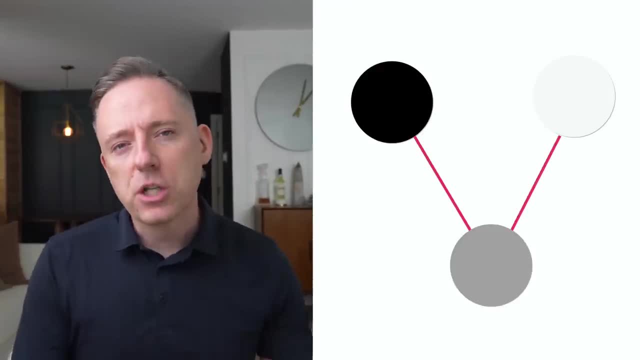 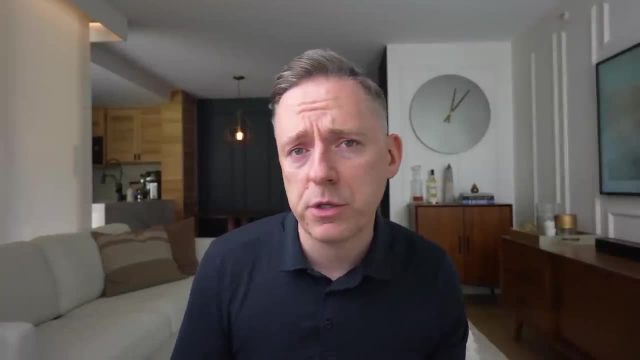 color is a mix of black and white, but actually in design, gray can be mixed with all sorts of different colors And you can start to get something that resembles gray that maybe has a blue undertone to it, Something like thundercloud gray You can see here. this is gray but has a 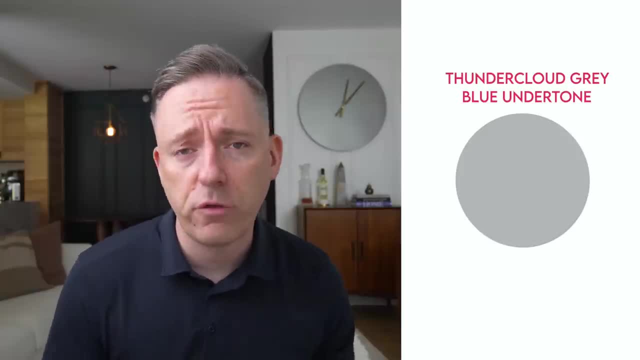 little bit of a bluey sort of tone to it. This is what I think a lot of people think of when they think of gray. This was what was really popular several years back, something like this- And again I'm going to use paint colors as an example here- by Benjamin Moore, but honestly, you could 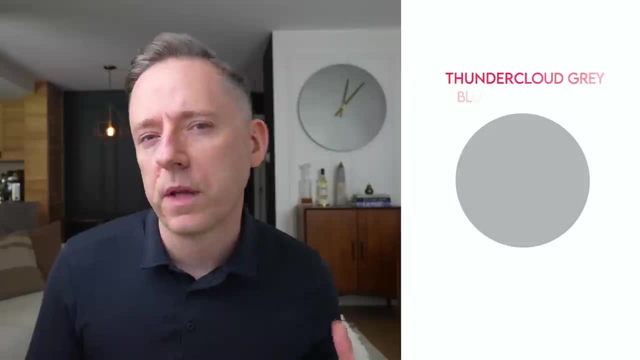 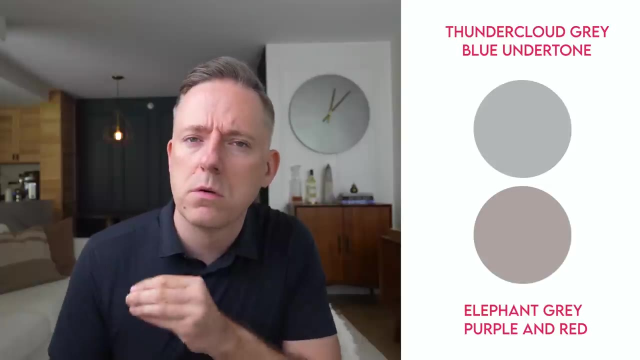 just apply this to all sorts of different decor and whatever. We're really just talking about the color theory here. Now compare that to something like elephant gray, which is going to be a little bit more violet. It's going to have a little bit more of those purple undertones, a little bit more red. there It's. 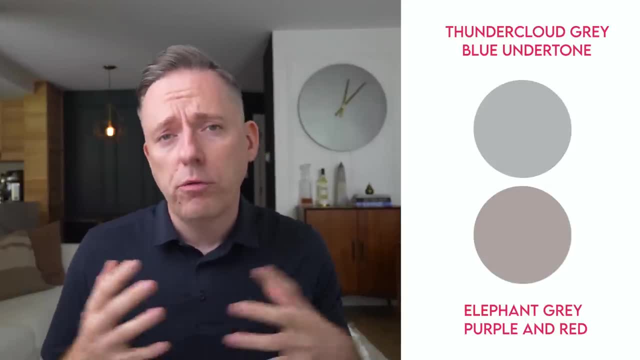 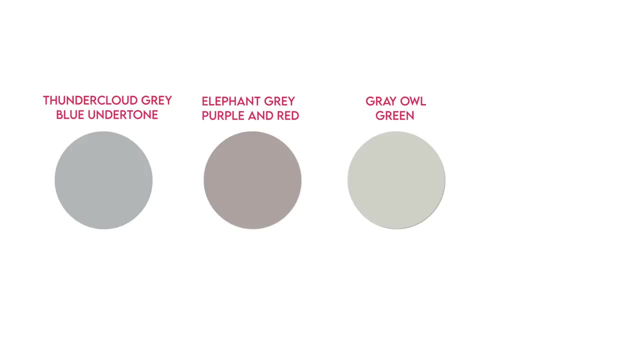 going to kind of warm it up a little bit. It's still gray, It's still going to read as gray on your walls to a certain degree, but you can see it has a very different undertone to it Now. take something like gray owl- similar story, except it's going to have a little bit more of a green. 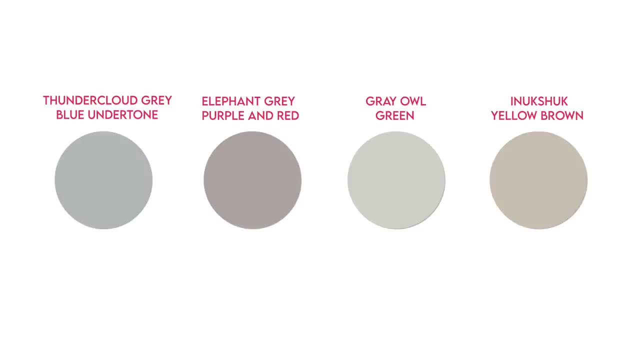 undertone to it And a nook shook has something of a little bit more of kind of a yellow brown undertone. So you can see it's still under sort of this general umbrella of gray, but it's going to read as very different depending on the undertone. 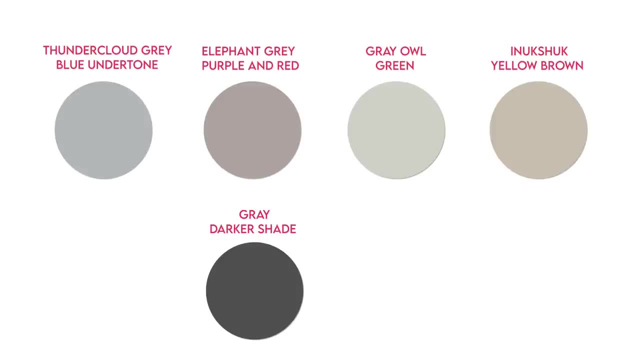 Tones that you might have. And, of course, if you take gray but then add more black, you might get something like gray. or if you add more white, you're going to get something like classic gray, which is arguably actually more of an off white. So all this is to say gray is actually a lot more. 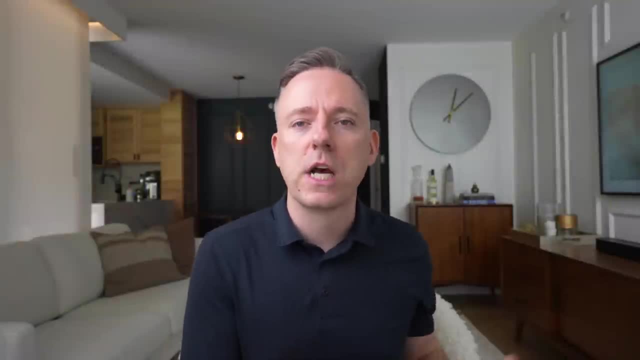 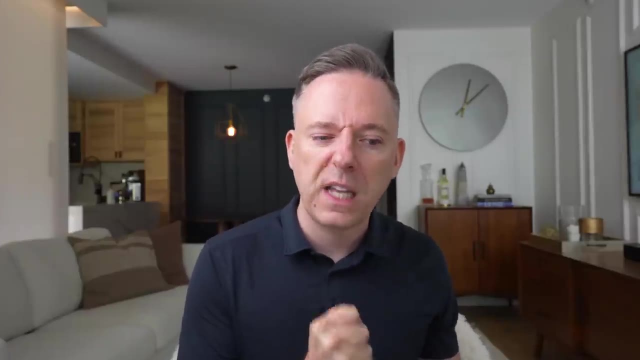 complex and it's not inherently a bad color. It's actually a very important color in interior design. I think it was a particular style of gray that was so popular for so many years that kind of had a lot of people feeling like it read as really gray and depressing, especially because it had so 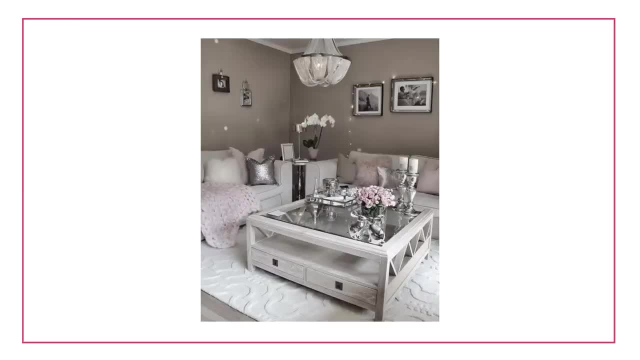 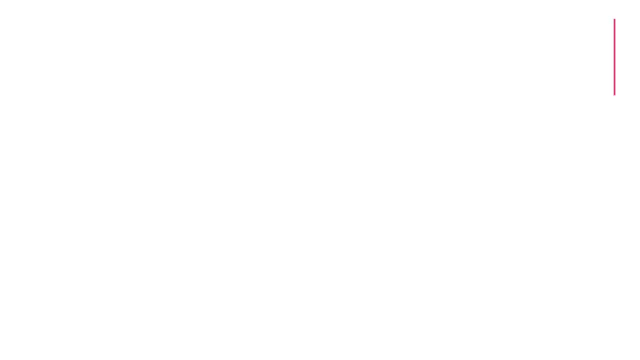 much blue added to it And it was a lot of those blues and silvers with chrome accents, mirrored finishes and rhinestones and glam And it was all that sort of style of gray that was really popular, that I think we have really shifted away from an interior design towards something a 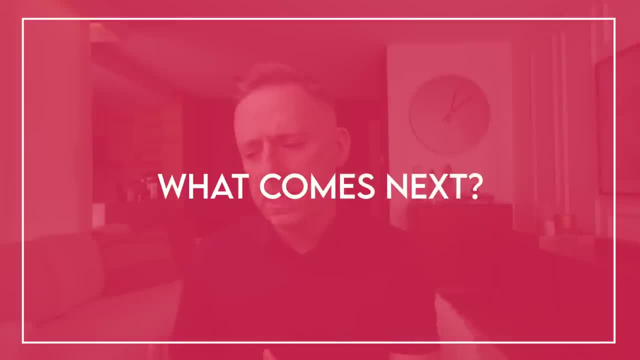 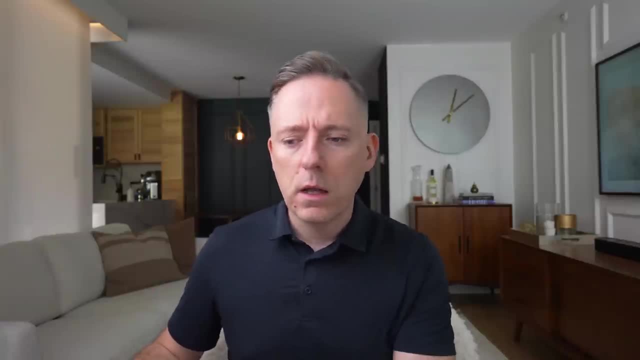 little bit newer. So let's talk about what comes next, right? So what has happened in interior design, in home decor, that has had us all sort of moving away from gray, and where are we going and why are we headed there? Well, first of all, let's just get this out of the way: If you love gray and 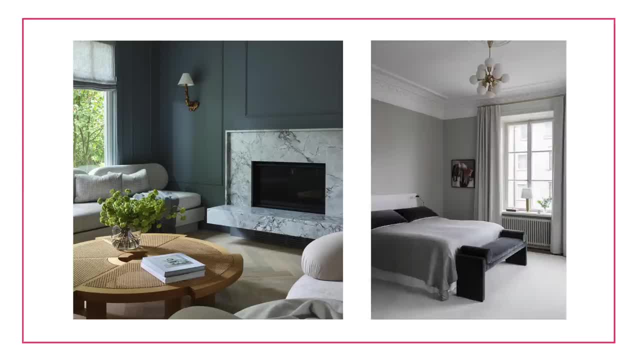 you still love all these images that I'm showing and your home is gray and you have the gray flooring and you still love it. don't listen to me. I'm just a guy on the internet Like this is all for the learning. You don't have to change that. No one is making you paint your home. 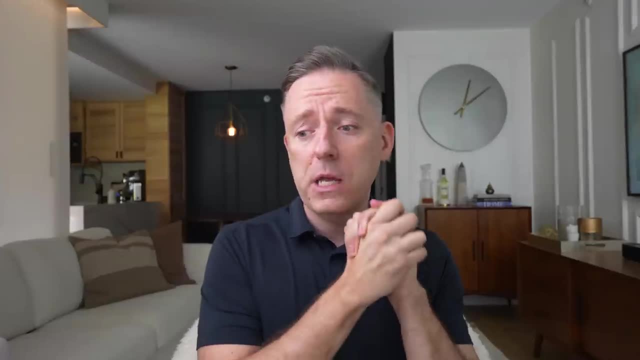 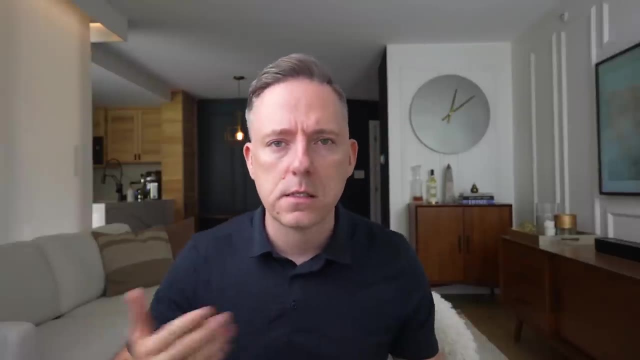 You can absolutely do whatever you like here. There is no question here. But you will start to notice that you will see some changes showing up in the different retailers that you might like to shop at, because as they are adjusting to trends and styles, so will the products that are in their 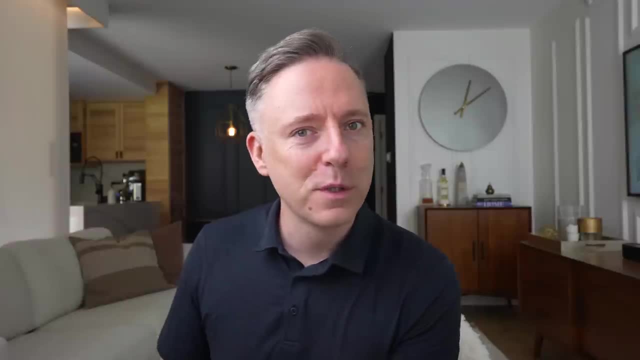 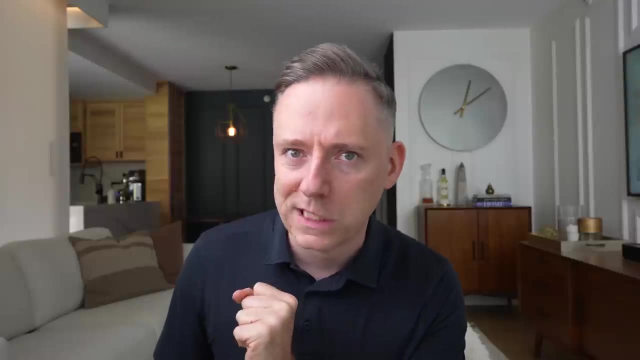 showrooms. So something to consider. if you see all these new tones that are popping up, that's going to be why. So where is design headed? Well, for several years now, I think, due to the fact that we were all stuck at home for several years, I think that design has really headed into a much 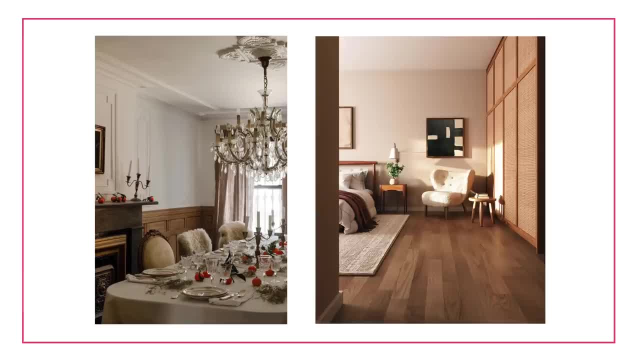 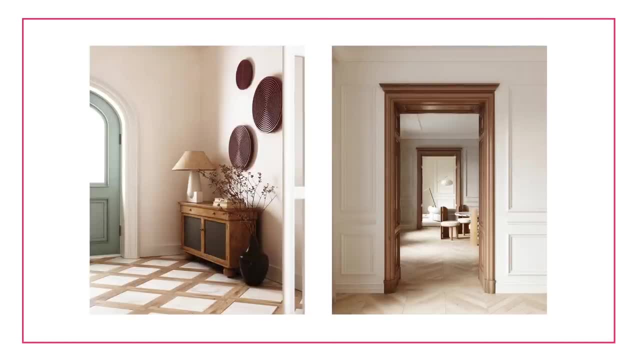 warmer direction, And those cooler blue-gray tones have been replaced with something more like beige and cream and moving in that warmer sort of color palette. Now the neutrals, the true neutrals to me, are white, black and gray. But beige is an interesting one, right, Because it's in wood and 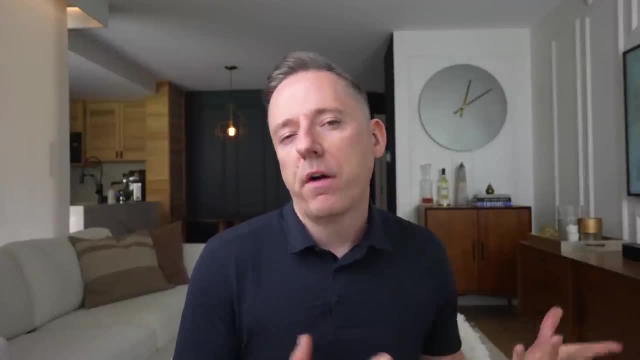 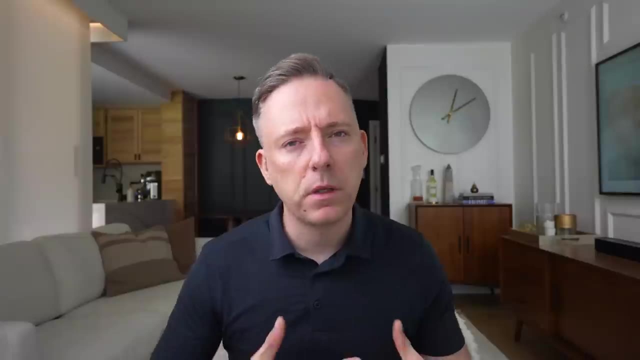 it's in, you know, different natural materials. it can sort of read very much like a neutral. So usually in design we put beiges and creams and things in sort of the neutral category. Because they are. they typically go with a lot of different things, but actually really it's a. 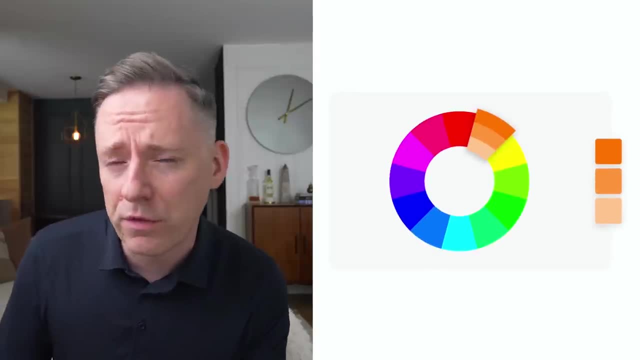 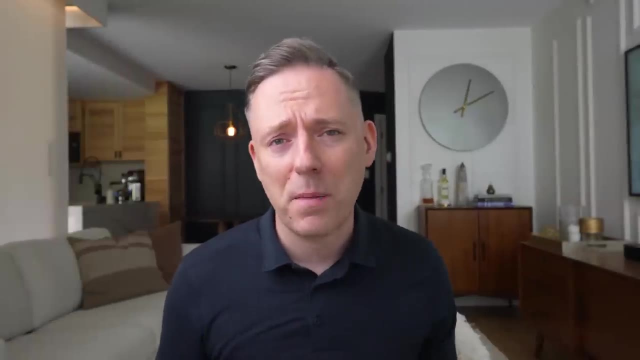 subsection of brown, which sits more in kind of the orangey area of the color wheel, rather than the black, white, gray, which to me are more sort of true neutrals in that sense. So design trends oftentimes work in a pendulum and sort of: you see, this swings right. We had, like you know, 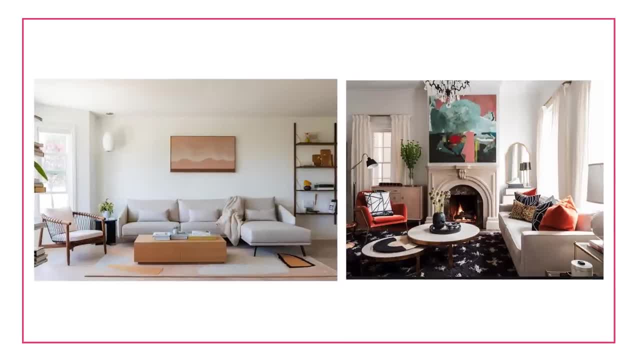 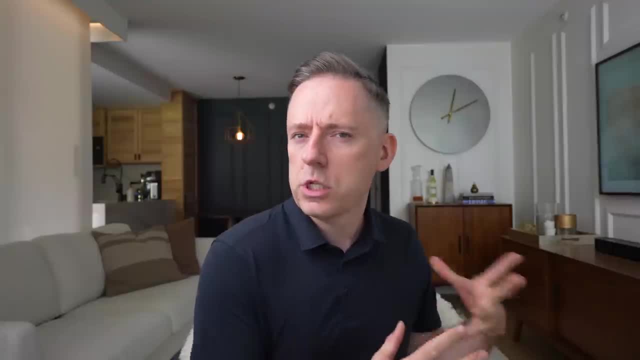 minimalism for a while and then maximalism, And now we're going to go back to minimalism, probably in several years, right? So the same is true for neutrals and pink colors. So gray felt very cold, felt a little bit sophisticated and cool and chic, but it also felt really sort of standoffish. 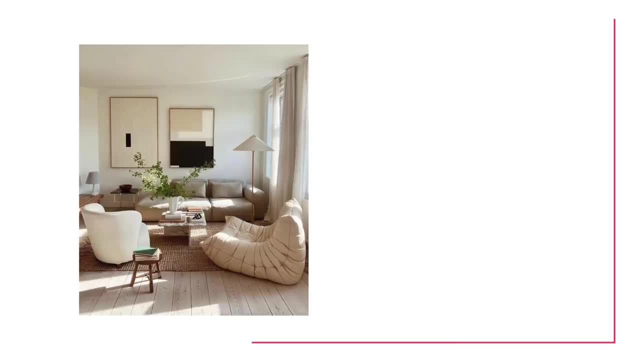 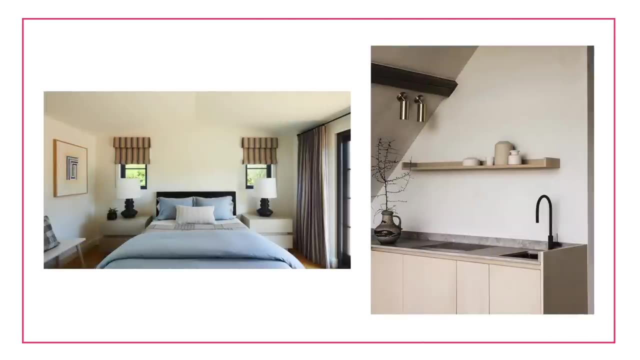 And so this movement towards beige or cream and sort of, in this sort of warmer area of the color palette, still going to feel very neutral, but it's going to feel a lot more friendly and a little bit more homey for people And that's why we're seeing so much more movement towards these. 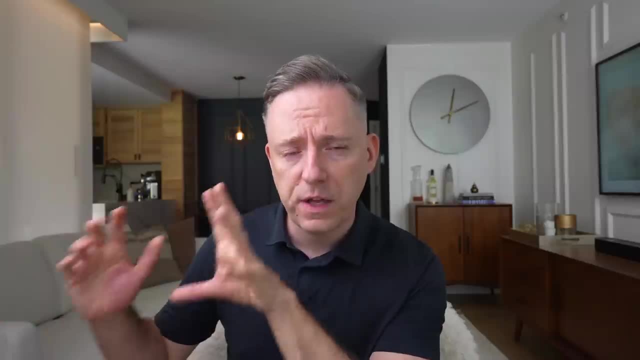 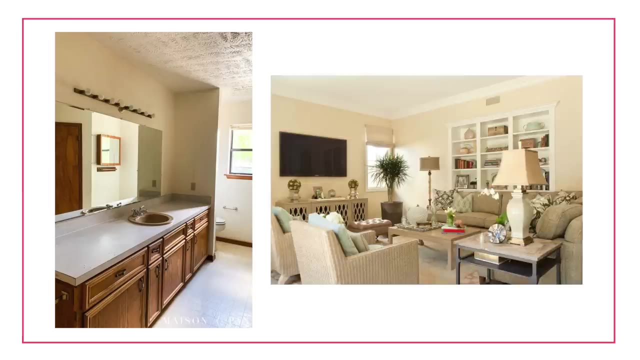 tones. Now if you have some nineties PTSD of the suffocating all beige bland room, I hear you. I get it. I do as well. I think it's being done in slightly different ways than it was back then. A lot of the pink colors, the sort of backdrop of the space is going to lean a lot more. 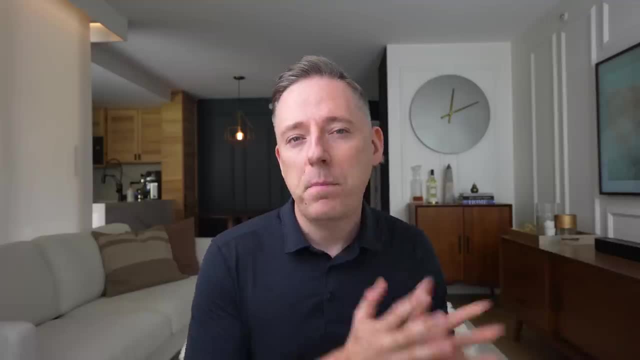 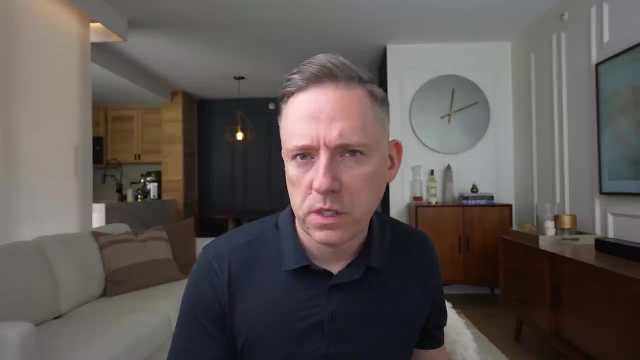 kind of like a white or an off-white or maybe even something like a cream and beige and browns are being sort of brought in more in furniture pieces and decor items, And of course those gorgeous wood tones and things that were that we're seeing all over the place. That is just. 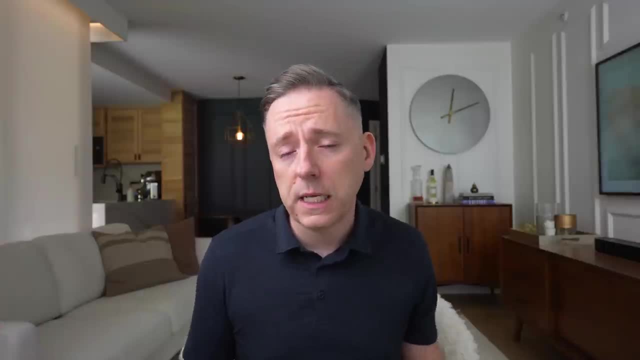 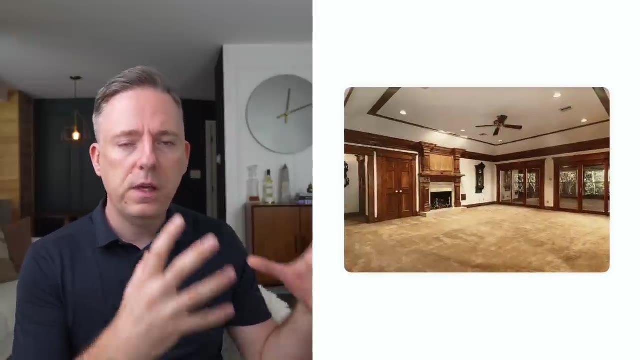 always a natural, timeless material that you're going to see all the time, because wood naturally leans, warm and therefore fits really well into this style. So I would say that the nineties really heavy beige, all beige palette, where everything felt really. one note is not the 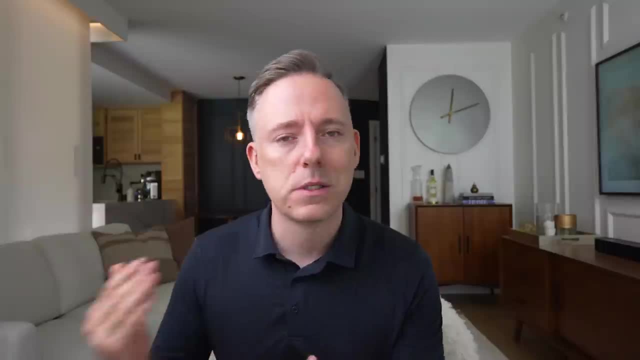 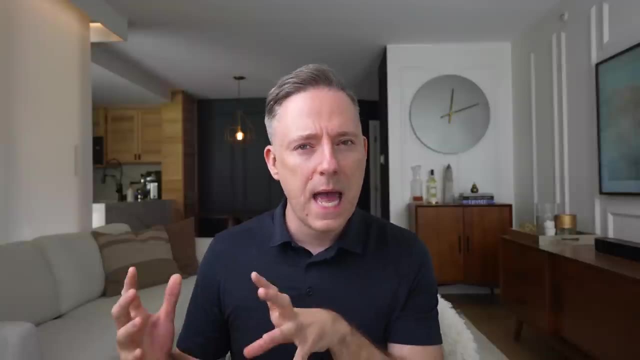 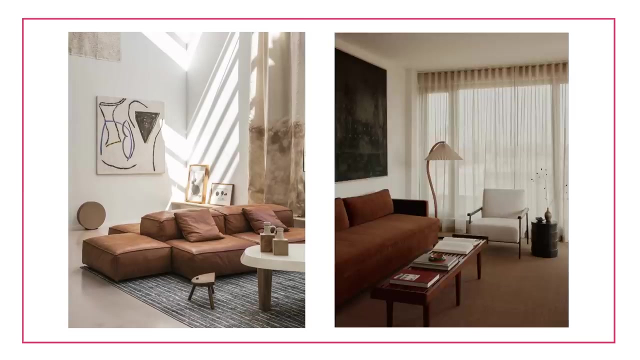 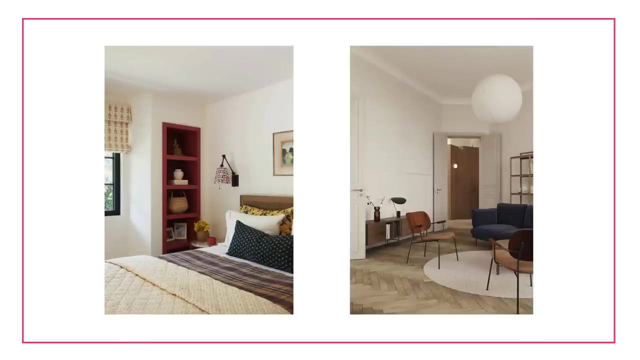 direction that it's headed. Instead, it's kind of like a white or an off-white or maybe even something that's a little bit more light and airy, because you've got lots of different contrasts happening even within beige and cream and brown. It's playing with that contrast of those different. 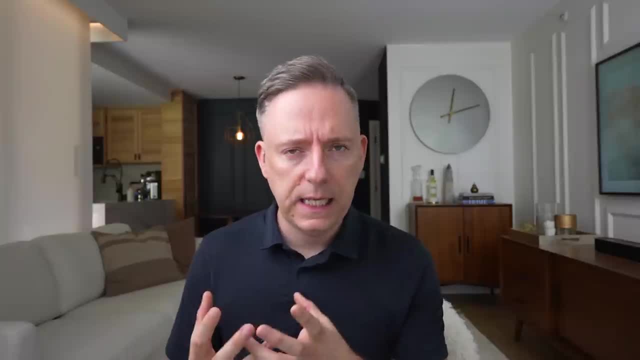 areas of brown. that I think is really key Here to nailing this look, so that you don't get a space that just sort of feels very. one note, which was sort of the popular thing that we saw the last time: beige was really popular. 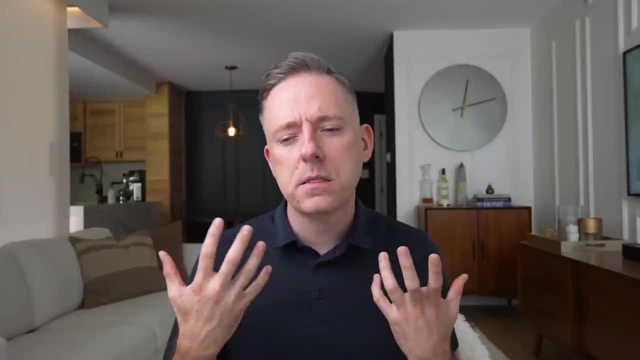 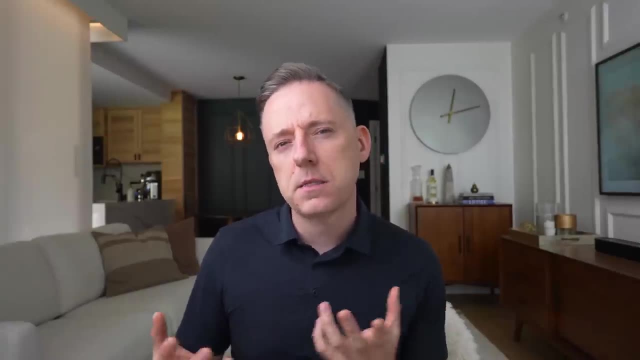 I think this makes beige feel a lot more sophisticated and it makes it feel a lot more nuanced, because beige- let's face it- is sort of synonymous with boring And I understand that, but it doesn't necessarily have to feel that way, I think, if you're playing with lots. 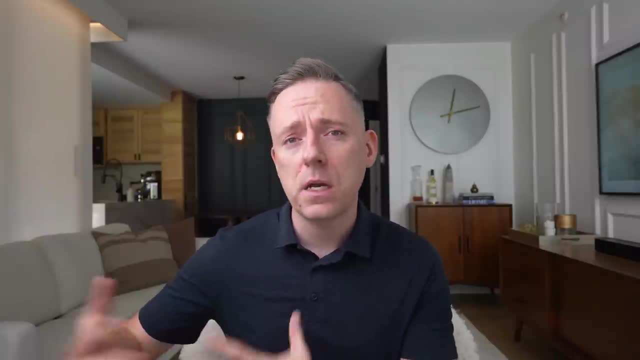 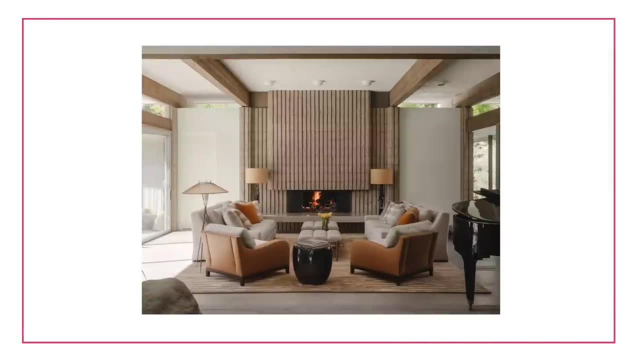 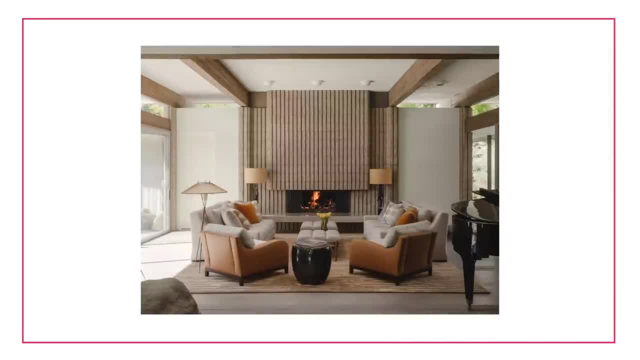 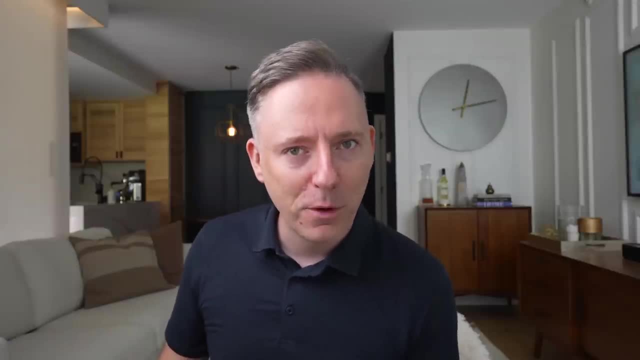 deco space You're not going to get, you know, crazy, uh, necessarily like crazy maximalist spaces which I know a lot of people are loving right now. but within the neutral realm, if that's what you love about your, you know, in a home this can feel a little bit more fun than what. 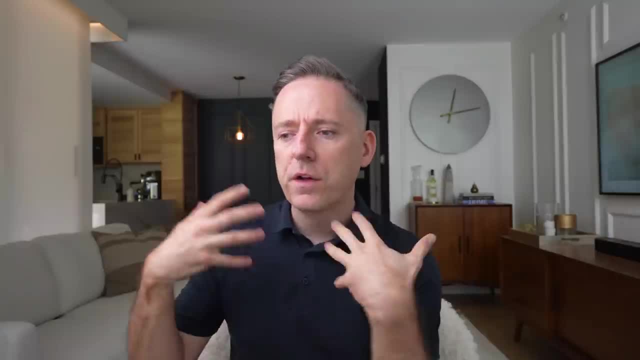 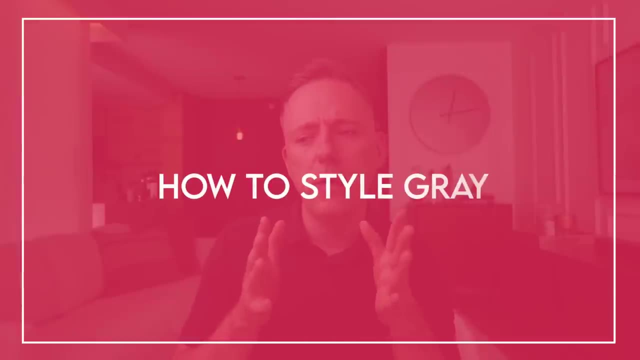 you're going to get with. obviously, compared to those other styles, not so much, but it's going to feel a little bit warmer and comfortable, which I think is what a lot of people are really looking for in their home. Okay, So now let's talk about, for a second here, what if you have a lot of gray. 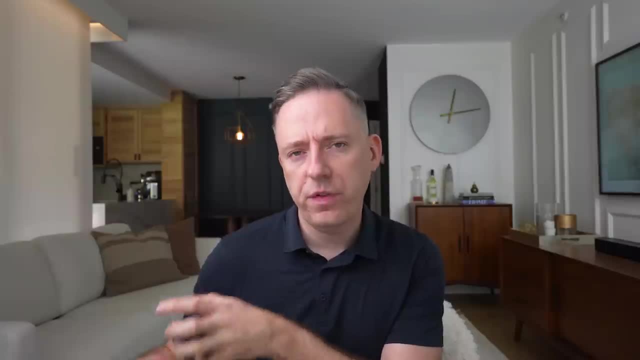 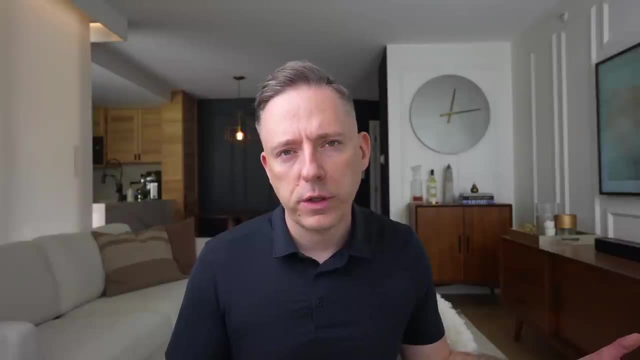 in your space and you're thinking: well, how can I update with this sort of new, warmer direction that is so popular, without necessarily ripping out all of that sort of gray engineered hardwood that I put back in 2016.. And I'm not really ready to get rid of, nor can I afford to get rid of it? 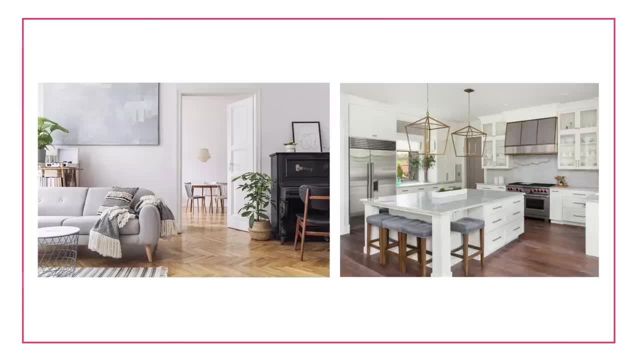 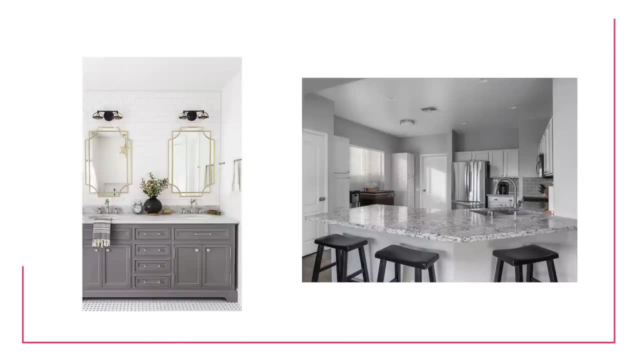 because, let's be honest, if we just sat and shake, it's not practical for most people to chase every single trend, especially when we're talking about fixed elements, when we're talking about flooring, we're talking about tile. It's really difficult to swap those things out for the new trendy color. 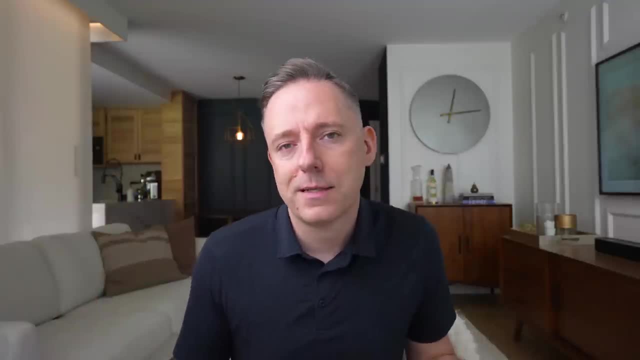 that this guy on YouTube Is telling you is a thing right. Let's be honest, That's not practical. So what do you do if you've got those gray fixed elements and you're looking at warming them up? Well, I would say, doing just. 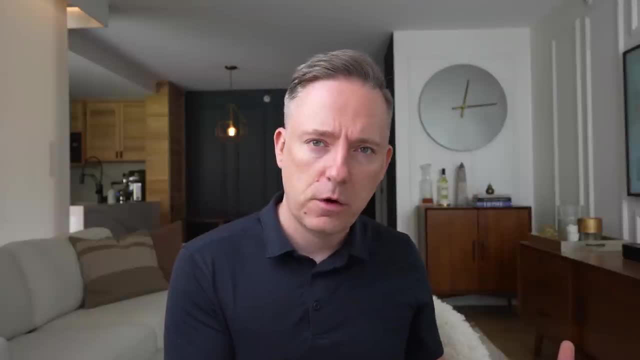 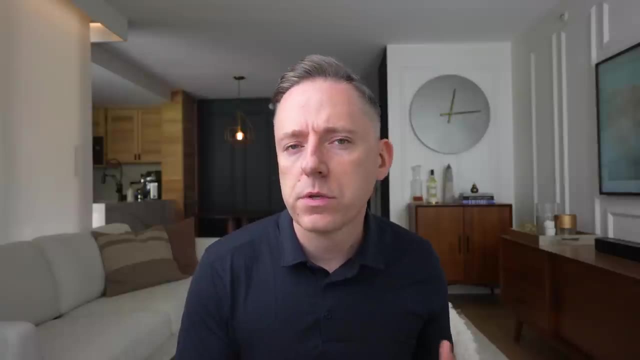 that using sort of yes, you might have those fixed elements in a gray, but playing with that contrast and bringing in some of those warmer woods and creams and browns and things like upholstery, things like you know, your window treatments, things like your couch, things like 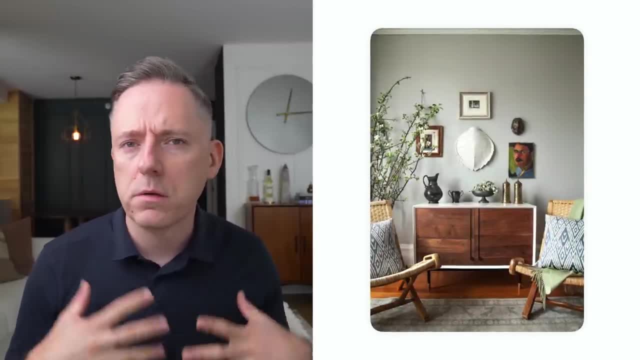 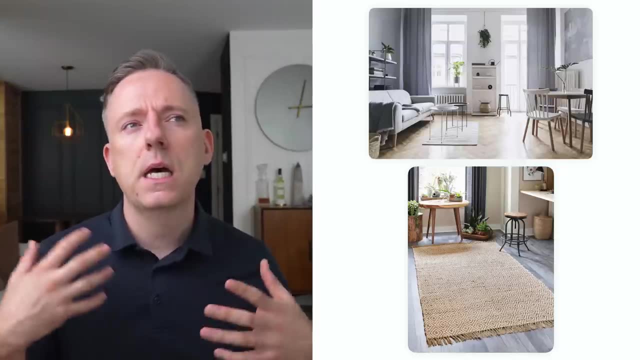 wood in your coffee table or inside tables. throws, pillows, all sorts of things like that, I think are really, really a great way to try to warm up a space and playing with that contrast a little bit. you know, take an interior design style like Japan. I love that style. What I think is so. 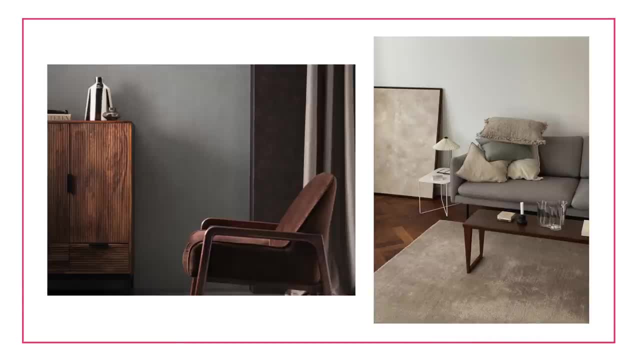 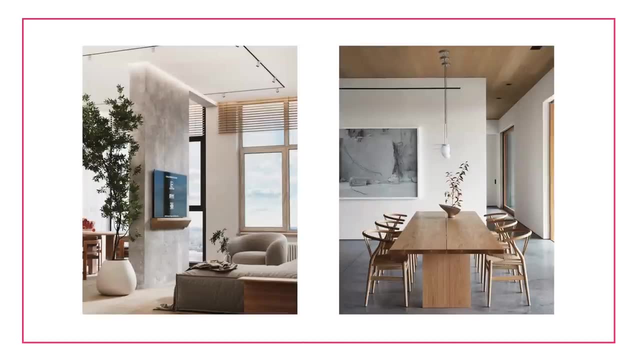 interesting about it is it does really play with the contrast between warm and cool. You'll see concrete floors and then you'll see sort of a wood coffee table over top And it looks beautiful because it's actually embracing the contrast between the warm and the cool. still feels very. 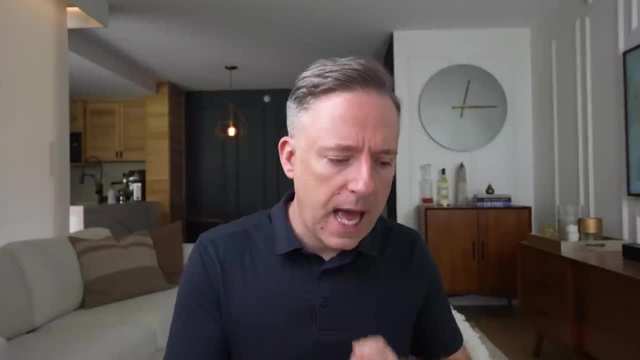 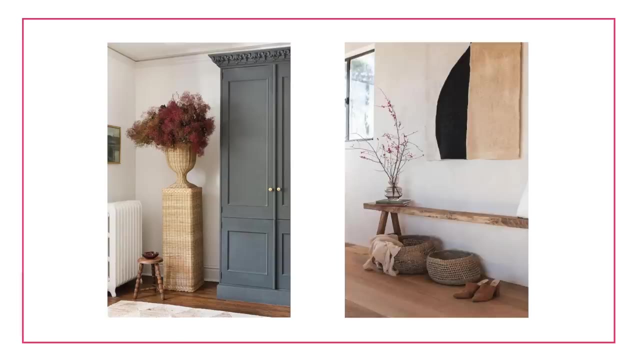 neutral but sort of has enough textural play and enough contrast to still keep it really fresh and interesting. So other ideas would be things like wicker baskets, you know wool throws and like a really gorgeous sort of camel color or a warmer beige tone, something like wood accents and things like. 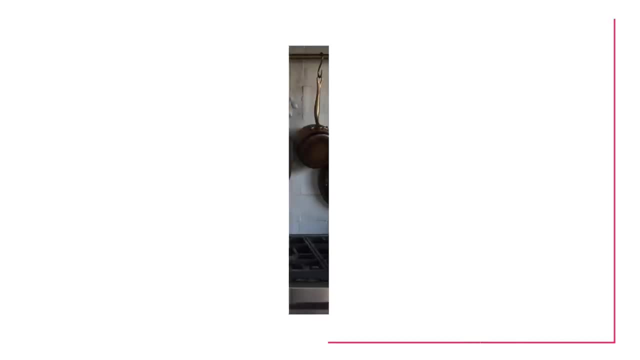 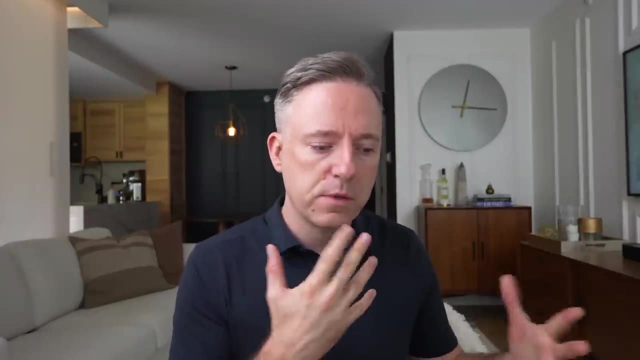 cutting boards or bowls or things that can really sort of contrast with maybe those cool gray quartz countertops that you have going on, you know. So consider if you know you're looking at some of those fixed elements being very, very gray and very cool. consider ways through your decor and 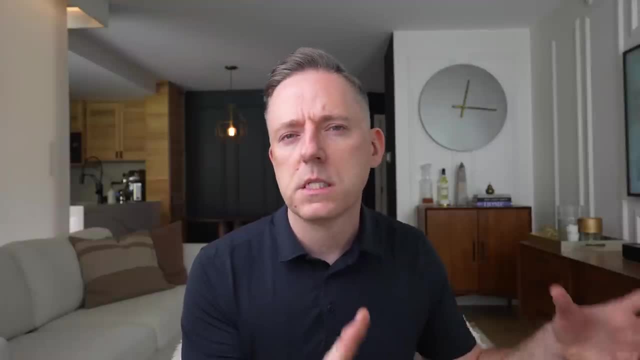 furniture that you're able to bring in some of those warmer elements especially, you know, if you're looking at some of those fixed elements being very, very gray and very cool in sort of these natural sort of materials that do such a really great job of warming up your space. 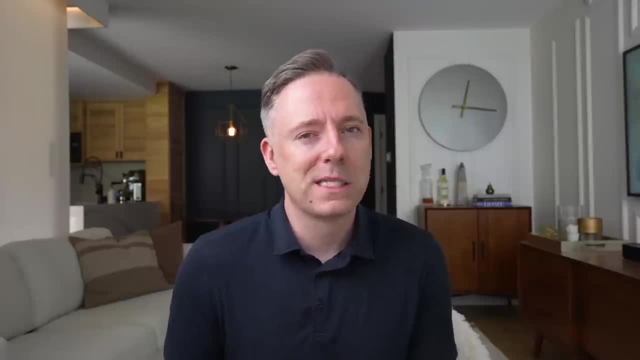 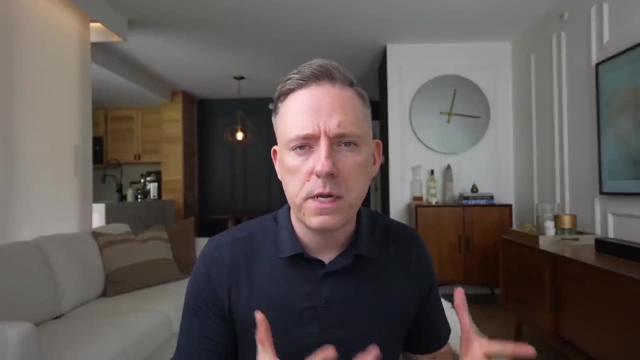 even if it leans really cool and you're thinking about playing with something in the warmer area of the color wheel, Also areas that you might also consider, things like rugs, bringing in those beige, creamy sort of rugs, especially in something like a natural material. It could be something like a. 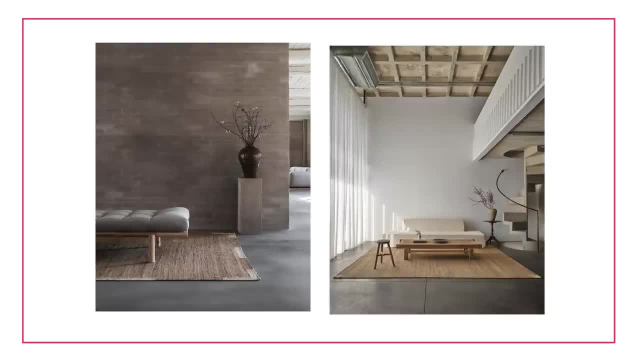 wool rug or something like a jute, something like that. but you're able to warm up some of those floors so they don't read quite as chilly as they necessarily might do right now. That can really work And also work your way up to the top of the floor. So if you're looking at something that's, 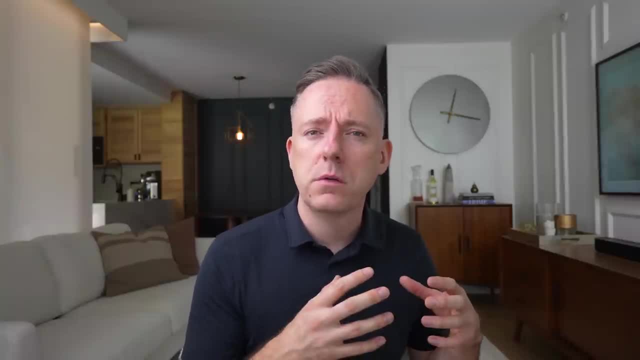 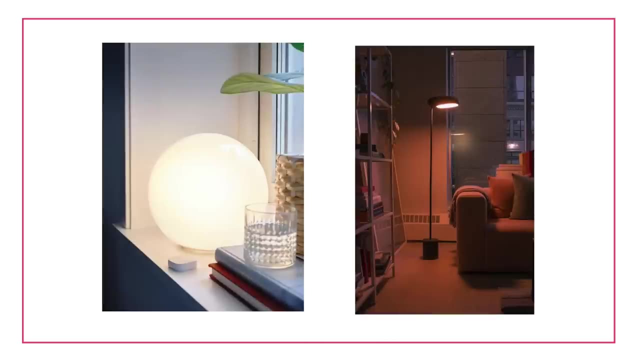 also working with lighting that's a little bit warmer in color temperature will also do a really good job of sort of giving a little bit more life to some of those gray walls or sort of gray accent that you have around your home, rather than going for those daylight bulbs or those really 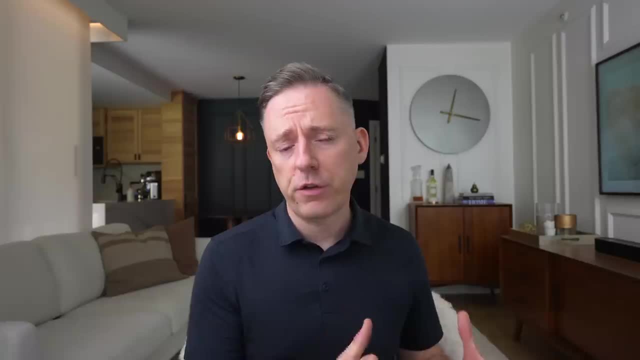 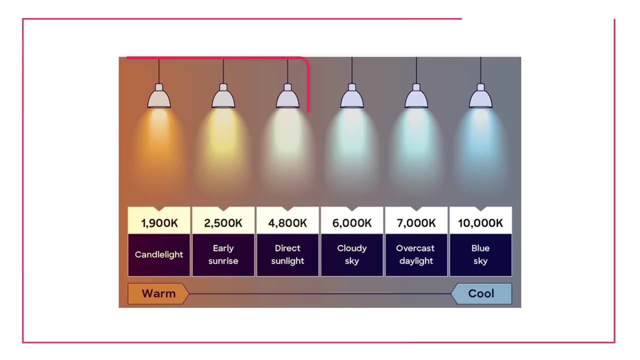 white lights that are just really going to make the gray feel even chillier than they already do because they are already in the kind of gray area of the color wheel. So working with something a little bit in a warmer color tone is going to really help warm up some of those pieces. And 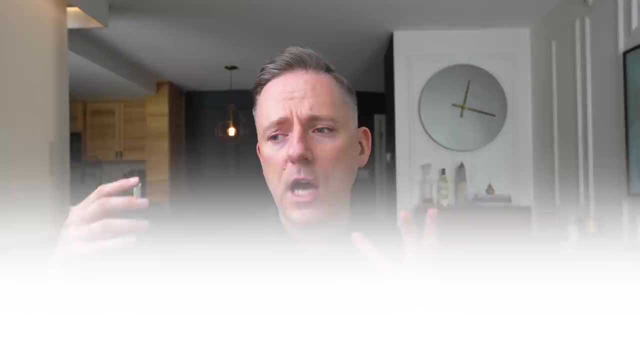 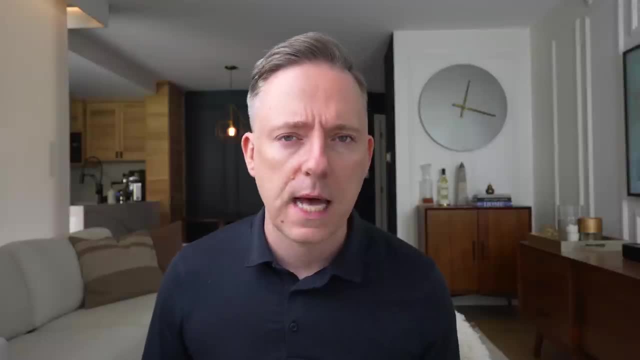 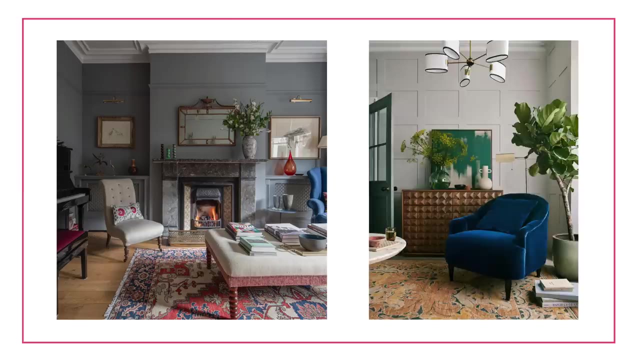 although that's kind of the point of this video, But don't forget that you can also, of course, add color if you want to. So if there are different colors on the warmer side that you're interested, maybe you're interested in playing more with oranges or yellows or reds or purples or something. 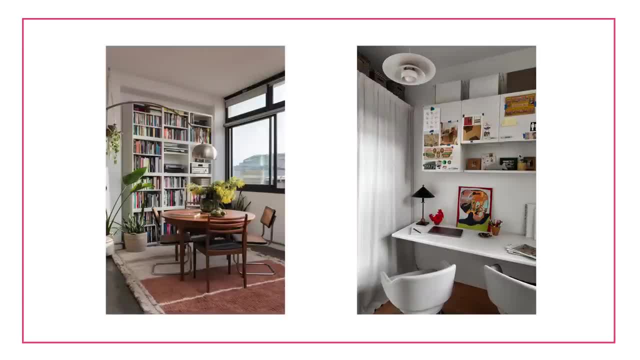 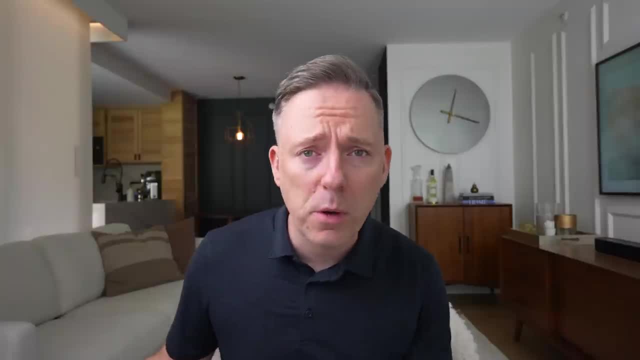 like that. that might be a great way, especially kind of those warmer kind of areas, to sort of warm up the space, make it feel a little bit more comfortable and have a little bit more fun than sort of the drab, gray spaces that we have seen in years past. You don't have to go brown or beige. 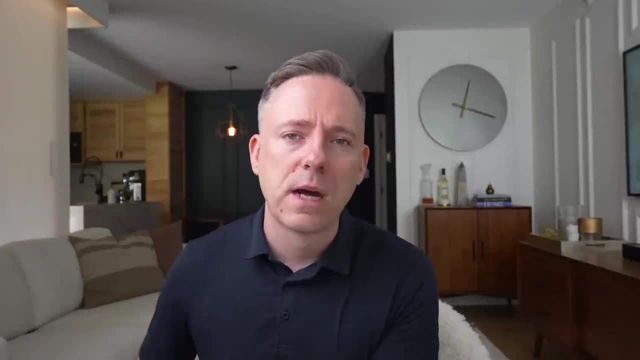 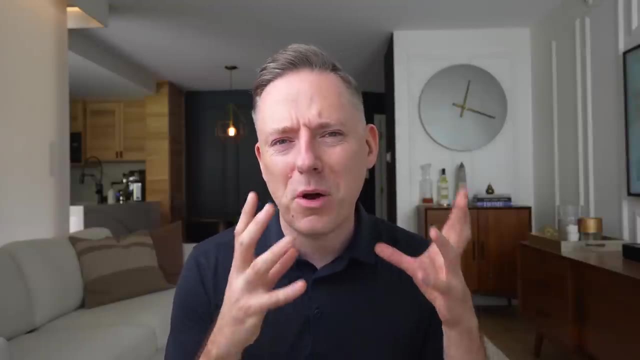 I'm just saying that, as far as neutrals go, that is the color direction that design has been headed the last couple of years And I don't really see that stopping for another several years yet. And also, by the way, don't sleep on texture. I mentioned it with the Japandi. 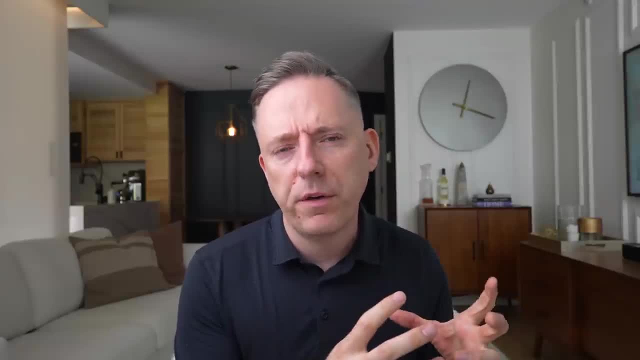 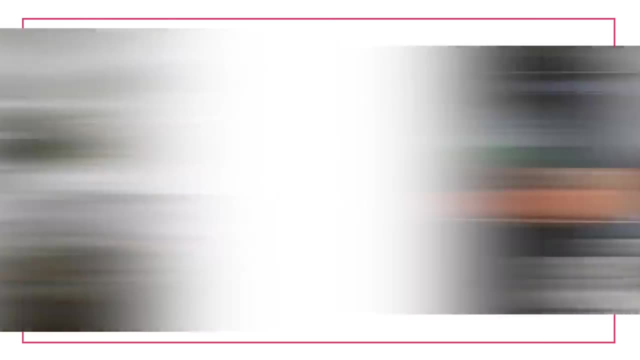 style, but adding texture into a space is really going to help it feel a little bit more comfortable. So those mirrored finishes that were really hard and sterile, consider swapping them out, even if you're not necessarily adding a whole ton of color. consider swapping them out for something. 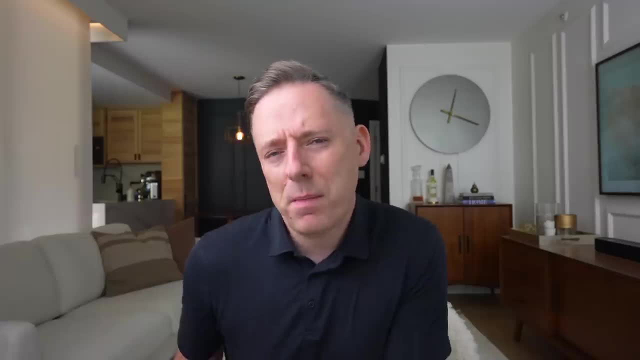 that's a little bit more natural and has a little bit more texture to it and maybe breathes a little bit more life into your space than you're going to get from something like a mirrored finish or a glass concoction. So that's a little bit more comfortable and maybe breathes a little bit more. 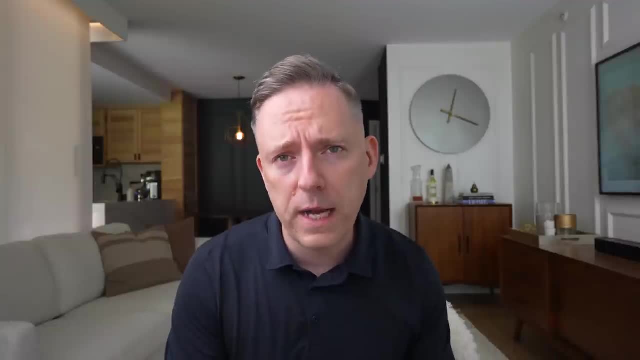 life into your space than you're going to get from something like a mirrored finish or a glass concoction coffee table or something like that. So those are my tips If you have a cool gray space and you're not quite ready to do like a full reno just because it's the new. 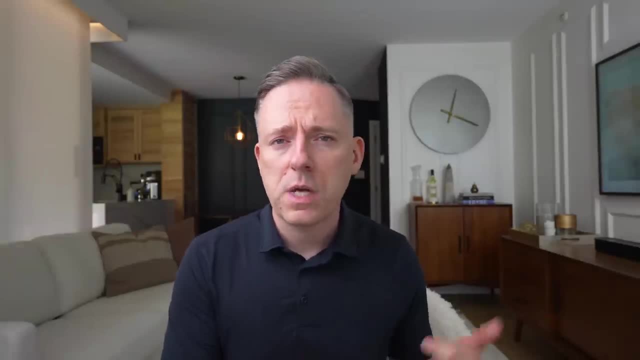 beige is the new flavor of the moment. things like paint, wood tones, color texture, all those things can really help a space feel more interesting. if you sort of have a gray space and you're thinking about kind of changing it up and making it a little bit more exciting, a little bit more. 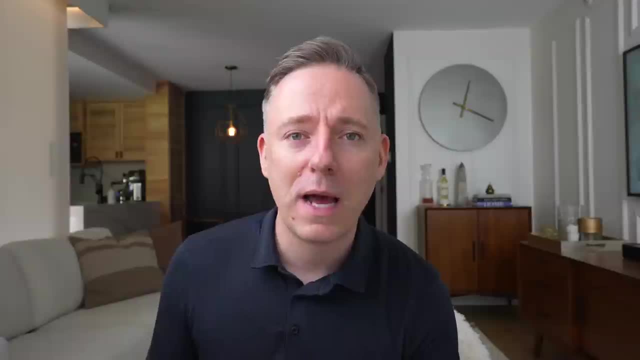 comfortable, even if you're not quite ready to say completely goodbye to gray quite yet. because you shouldn't, because there's nothing really wrong with gray, Like I said before, it's just you know. how do we find ways to make it a little bit more interesting and a bit more. 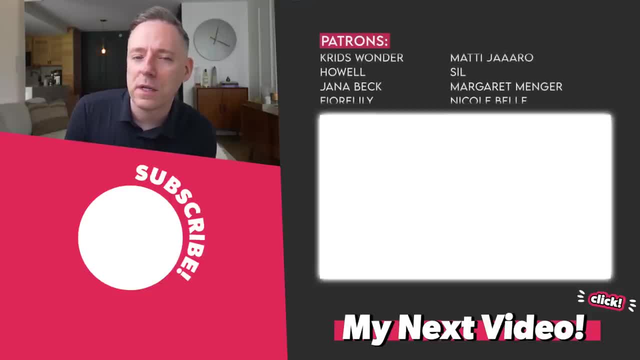 livable for most people. So that's it for me for today. you guys, I hope you really enjoyed this video. I will see you all next week Again. if you'd like to check out my course, check it out down in the description. I have worked on it for more months than I care to admit And it 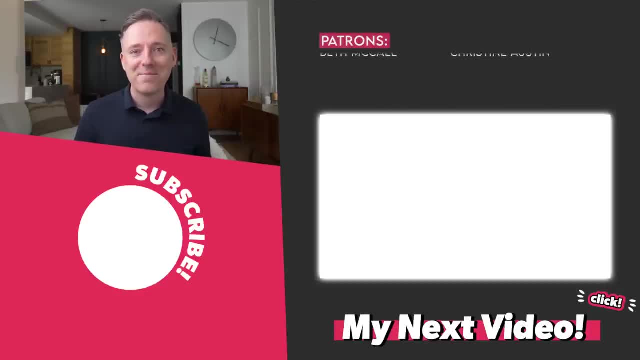 is now live, so you can go check that out And I'll see you on the next video. Thanks, Bye.